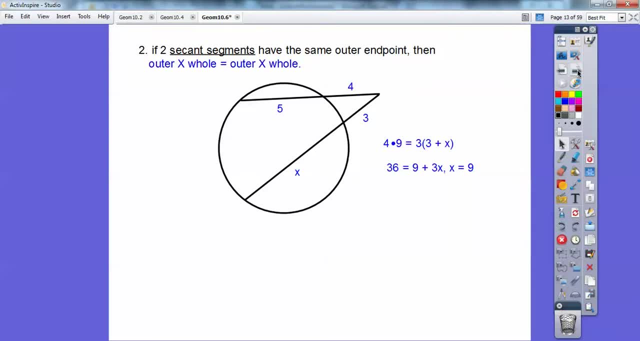 Okay. So, for example, if I had these numbers in here, I'm going to go this outer piece, which is 4 times the whole piece which is 9.. You see where that 9 came from. 4 plus 5 equals the other outer plus the other whole. 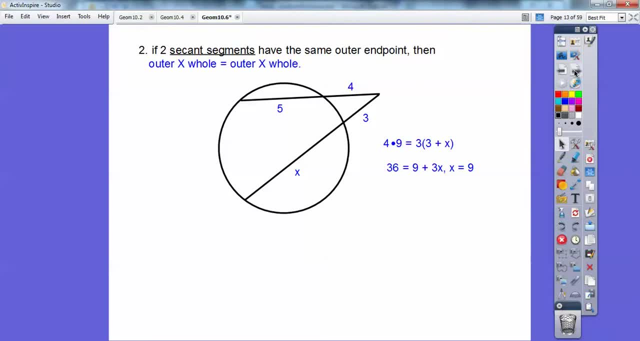 The other whole is 3 plus X. It's not 3X, you guys. Real common error. This is a common error. Don't do this Four times, or outer times inner, outer times inner. That won't work. 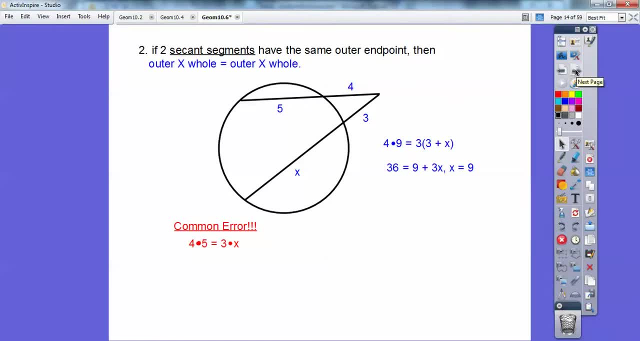 It has to be outer times whole, outer times, Outer times whole, just like the blue stuff right here. okay, All right. so if you have the same tangent segment and secant segment from the same outer endpoint, see how this tangent segment right here, this guy's a tangent segment and this. 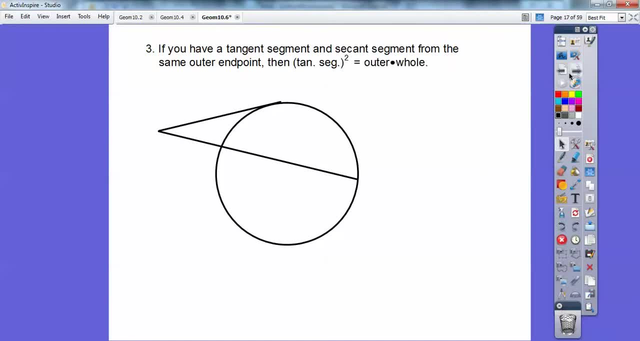 secant segment has the same outer endpoint, then it goes: tangent segment squared equals outer times whole. So for example, if I put some lengths in there, that's 24, 16, and X. so 24 squared equals 16.. 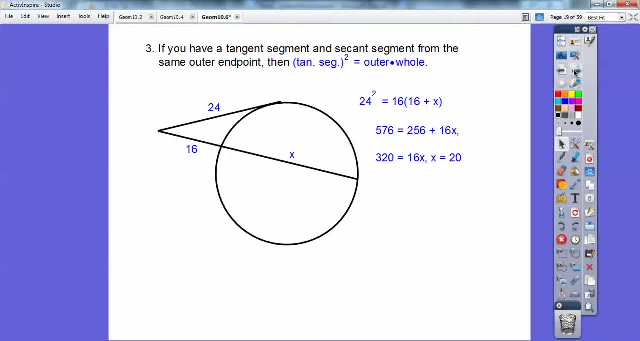 Don't forget, the whole length is 16 plus X, All right. and then you do your math and crank out and you get X equals 20, okay, 24 squared is 576.. So let's practice some of these, you guys. 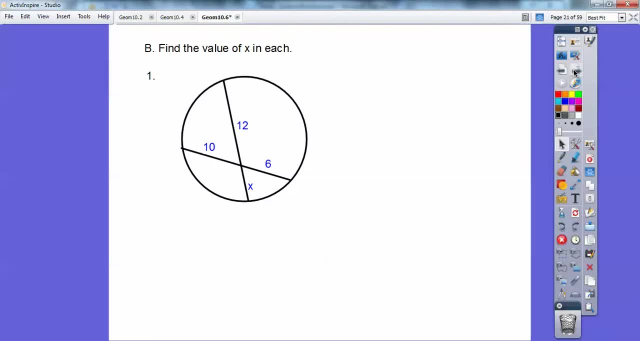 Find the value of X in each. okay, So here's two intersecting chords. So piece times piece equals piece times piece. So 12X equals 60, X equals 5.. Easy, huh? Okay, we'll get. let's see here's number two. 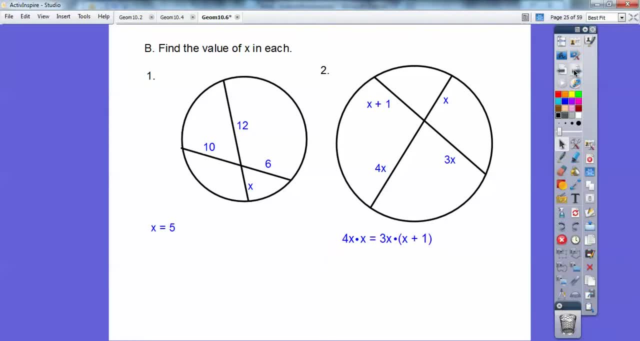 Piece times piece equals piece times piece. So 4X times X equals 3X times X plus X. Okay, Piece times piece piece times piece. 4X times X is 4X squared. and then, when you distribute, don't forget to distribute 3X through. 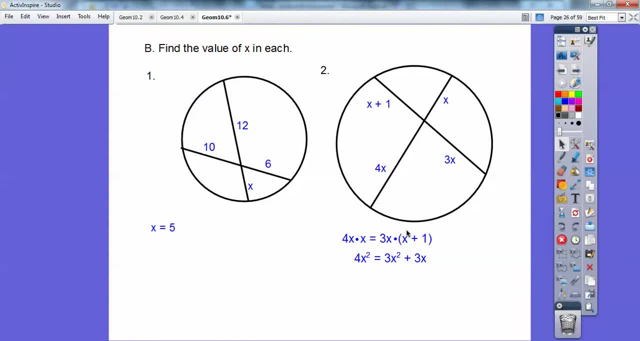 so you get: 3X times X is 3X squared, and then 3X times 1 is 3X. okay, So now we have a quadratic equation. so I'm going to subtract 3X on both sides and I'm 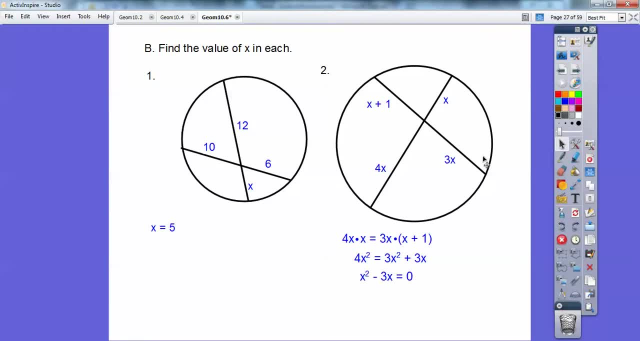 going to also subtract 3 on both sides Quadratic equations. we always want them equal to zero. So then we can factor this, We can GCF an X out of these two guys. I'm going to pull an X out of these two. 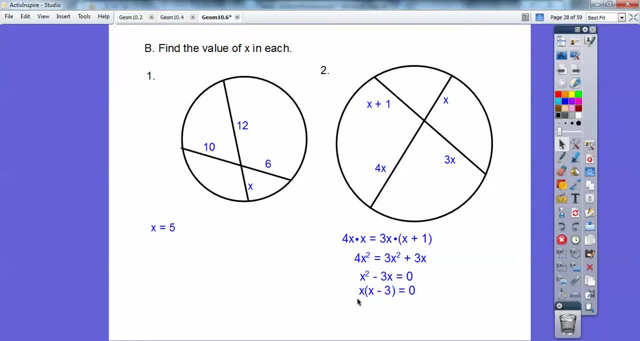 Okay, I'm going to pull an X out of both of those guys. There it is factored, Now it's called the zero product property. I can say: this factor X equals zero and this factor X minus 3 equals zero. So you get X equals zero or X equals 3.. 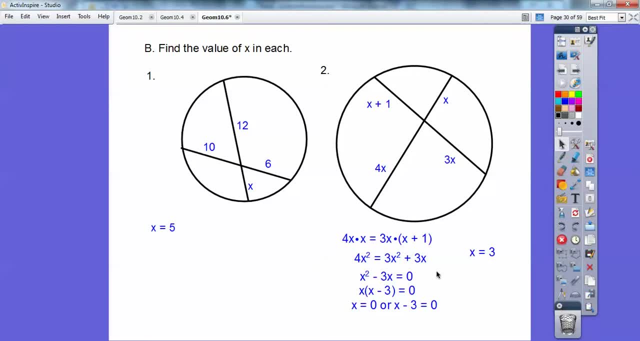 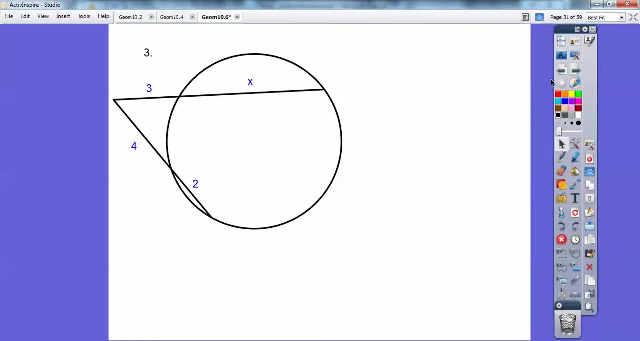 So you can't have a zero length, since X is talking about length. So I'm just going to go plus 3 plus 3 on this equation, so I get X equals 3.. Okay, All right. Okay, Outer times whole. 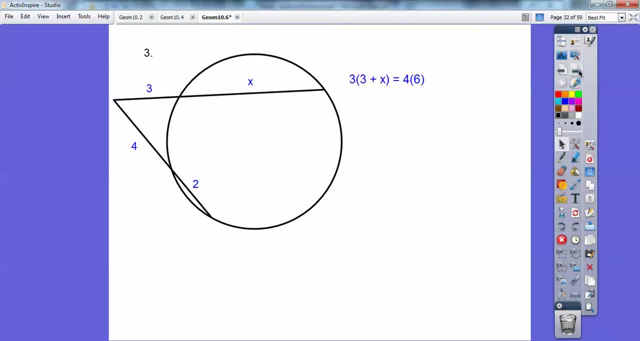 Outer times whole. So here we go. Three times 3 plus X equals 4 times 6.. Don't forget the 6 I got from adding 4 plus 2.. All right, Now I'm going fast. Remember you can pause and rewind. so I go fast to try and make these videos shorter. 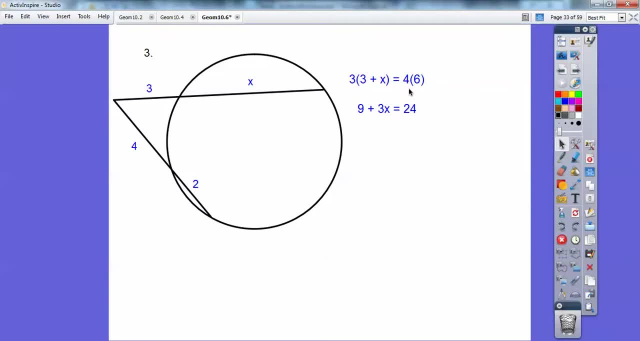 Okay, So distribute the 3 through 3 times 3, and then 3 times X, and then you get that equation Subtract 9.. You get 15X equals 5.. Okay, Outer times whole equals tangent segment squared. 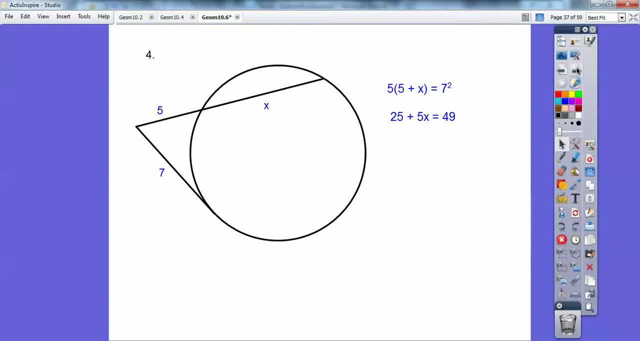 So 5 times 5 plus X equals 49,, 25, and then subtract 25 on both sides, You're going to get a fraction on that one. That's okay. So you get 24 fifths. Okay, Fractions are good, you guys. 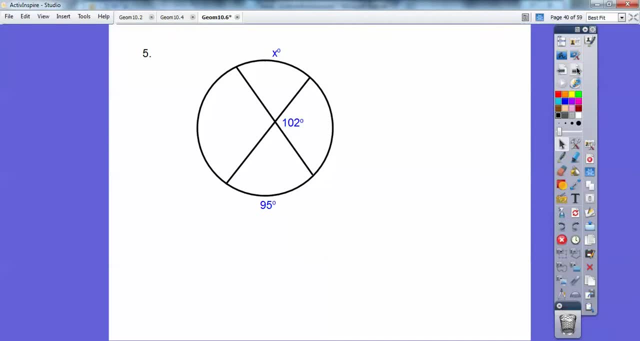 Don't be afraid of those. All right. So this is a review from a prior lesson that we did. you guys, What I'm going to do first is get that angle right there, that 78 degrees, because of that straight line, that red line is 180. 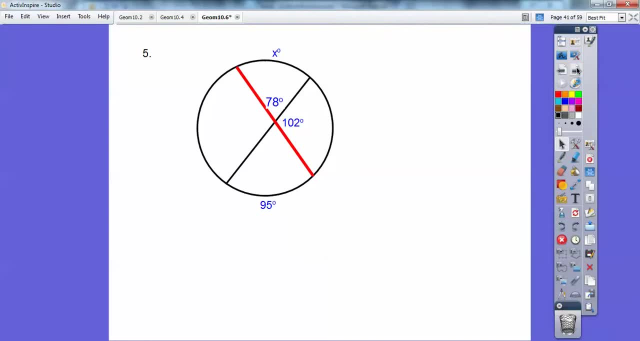 So I did 108, 180 minus 102.. Straight lines are great, you guys. 180 every time, And then that 78 equals half the sum of the intercepted arcs. So I'm going to add these two guys and take half of that. 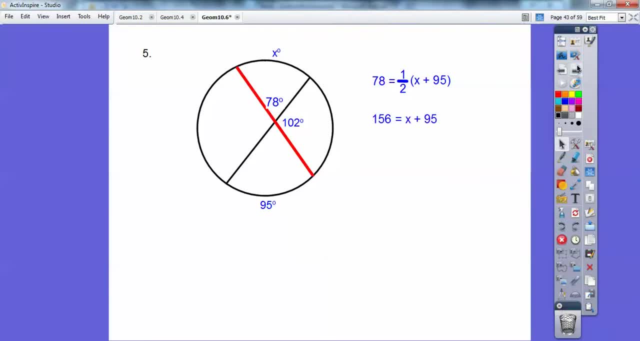 All right, And then. so I multiplied both sides by 2 to get rid of that half, And 156 equals X plus 95, then subtract 95 on both sides and you get 61.. Okay, Piece, times, piece, piece, times piece. 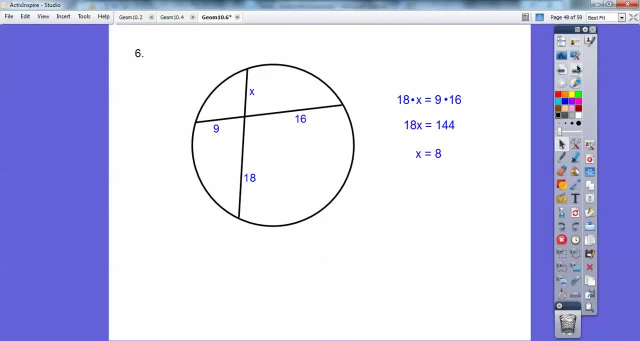 So 18 times X equals 9 times 16, 18 goes in 144, eight times Okay, Outer whole, outer whole. So here we go: Outer times whole equals outer times whole. Don't forget: the whole whole is X plus 29 and 18 plus 22..